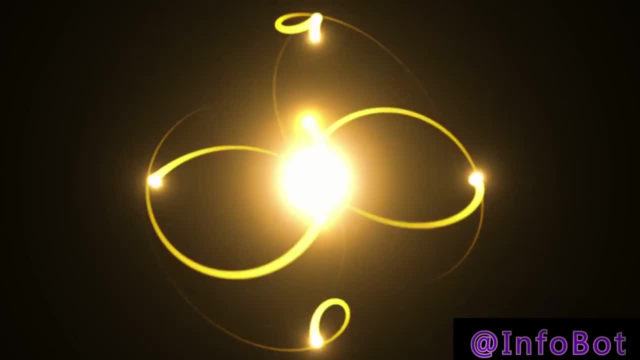 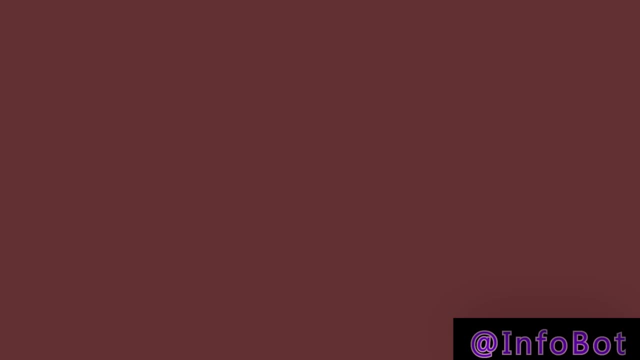 neutron. In the 1930s, physicist Enrico Fermi proposed the theory of beta decay, which helped to explain how certain subatomic particles change into other particles. During World War II, the development of the atomic bomb led to a significant increase in funding for nuclear physics research. 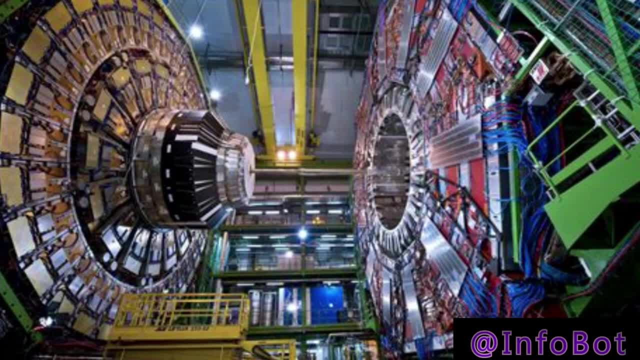 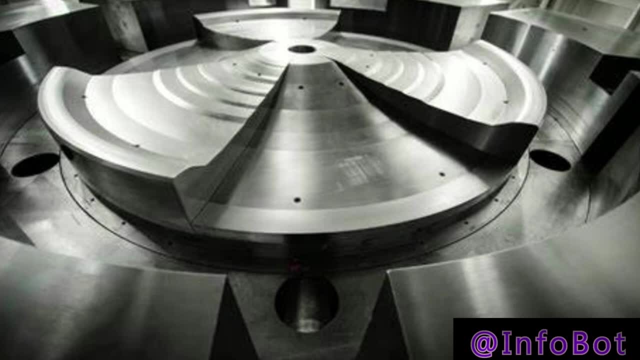 This in turn led to the construction of large particle accelerators such as the cyclotron, which allowed scientists to study the properties of subatomic particles in greater detail. In the 1950s and 60s, a number of new particles were discovered. 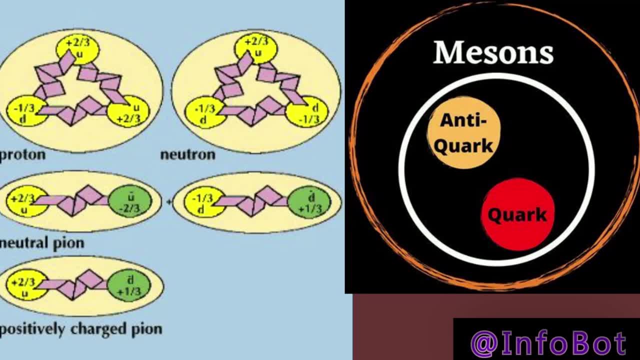 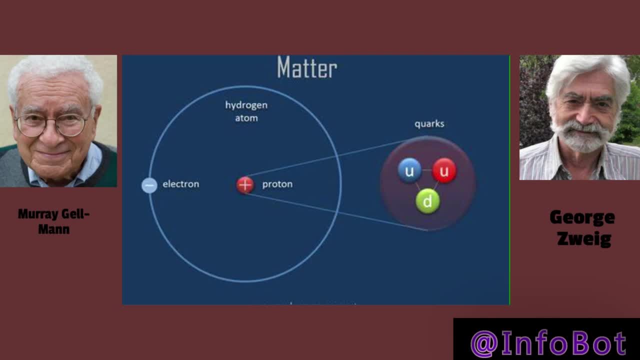 including the meson and the pion, which helped to establish the field of particle physics In the 1970s and 80s. the discovery of a new family of particles called quarks, proposed by JJ Thomson, was the first in the history of particle physics. 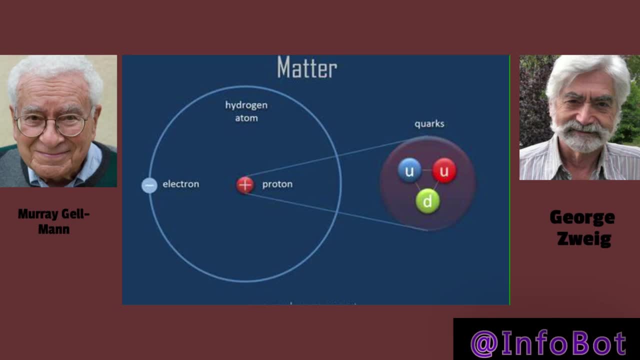 The discovery of quarks, which were developed by Murray Gellman and independently by George Zweig, which are the building blocks of protons and neutrons and other particles, led to the development of the theory of quantum chromodynamics, QCD, which explained the strong 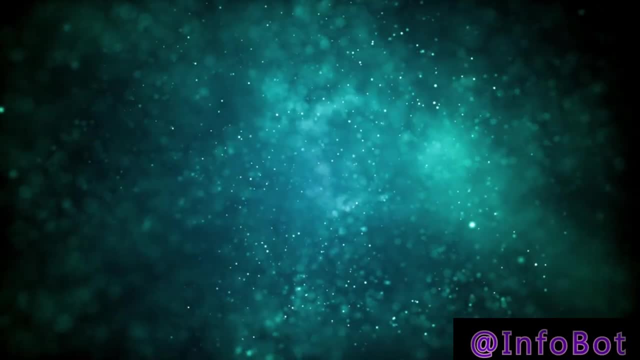 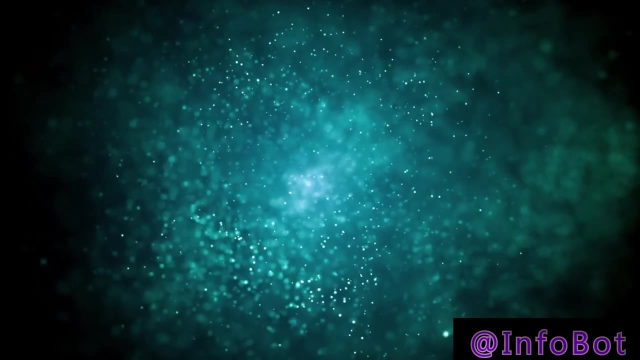 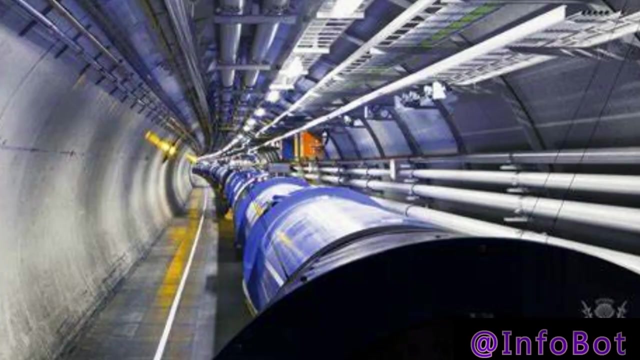 force. Nowadays, particle physics continues to be a very active field of research, with many ongoing experiments and projects aiming to understand the properties of subatomic particles and the fundamental laws that govern the universe. Particle physicists use high-energy accelerators to create and study these particles. 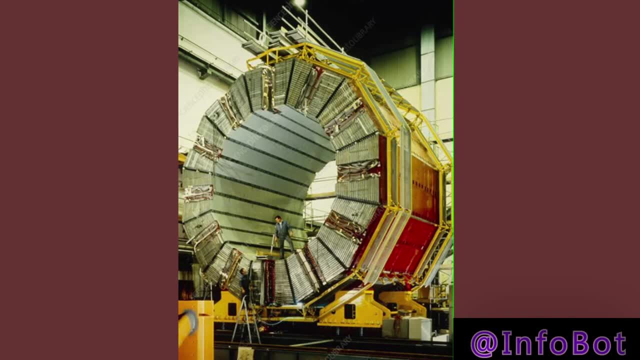 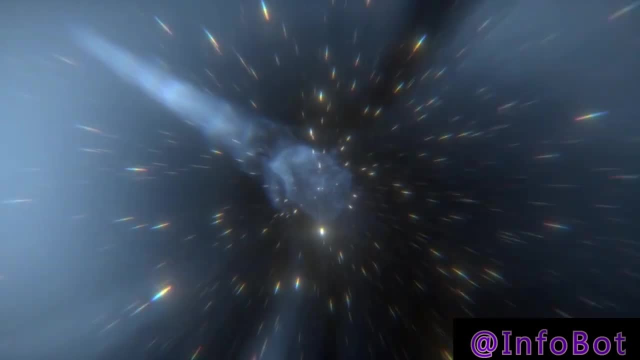 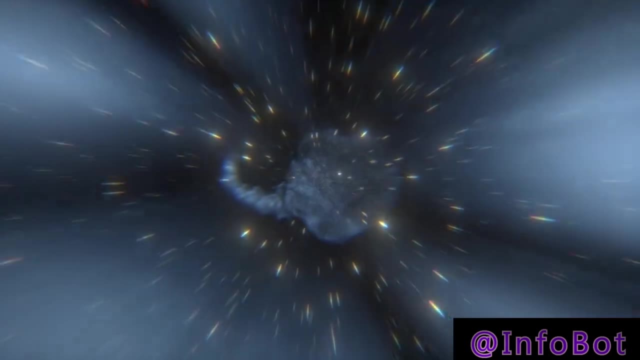 And they also use detectors to observe the particles produced by these accelerators. This helps them to understand how the universe works at its most fundamental level. By studying the properties of these particles, particle physicists are able to learn about the fundamental laws that govern the universe. They also have the hope to understand the nature of 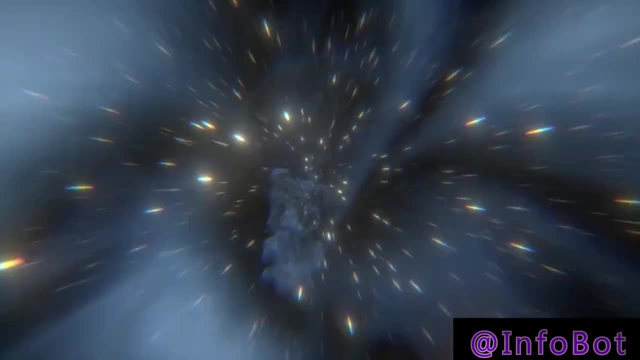 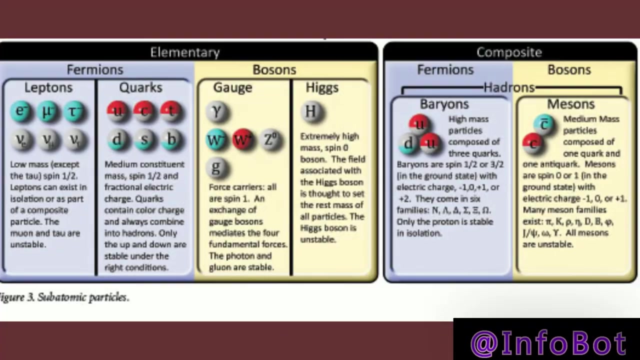 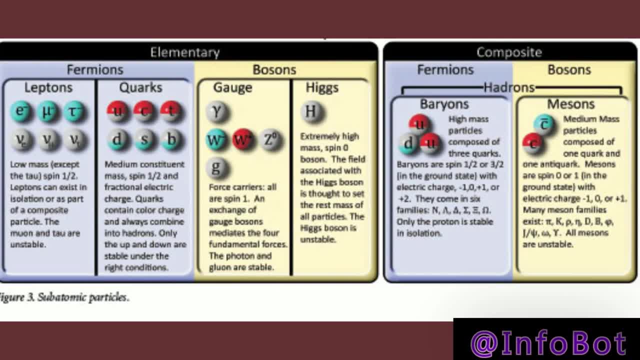 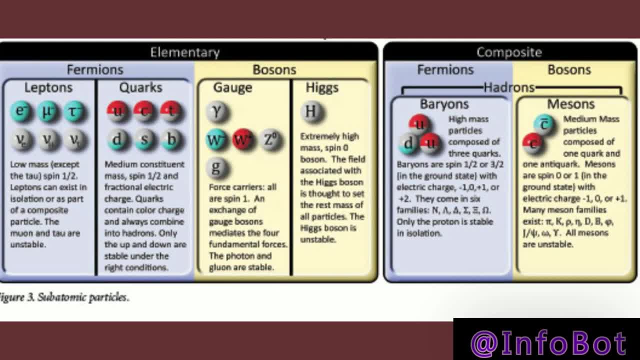 spin and obey the Pauli exclusion principle, meaning no two fermions can occupy the same quantum state simultaneously. Bosons, on the other hand, are particles that carry forces such as photons and the recently discovered Higgs boson. They have integer spin and can.